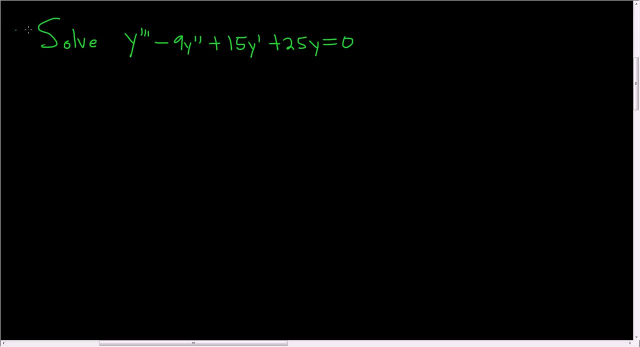 We have a linear differential equation with constant coefficients and it happens to be homogeneous because the right-hand side is equal to zero. Let's go ahead and solve this. We'll start by writing down the characteristic equation. So, because we have the third derivative, 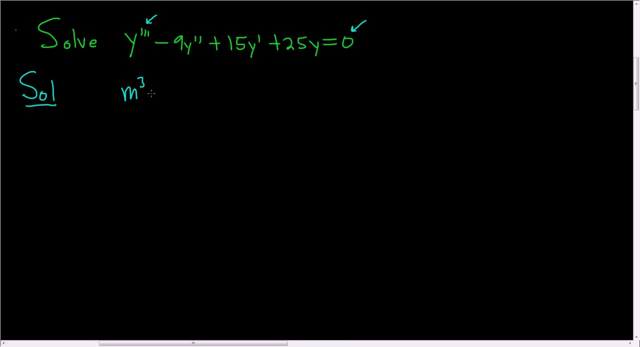 of y. here we'll write down m cubed and then minus nine. and then here we have the second derivative, so that's m squared and then plus 15.. Here we have the first derivative, so that's m. and then here we have the zeroth derivative, or just y, so 25, and this is equal to zero. 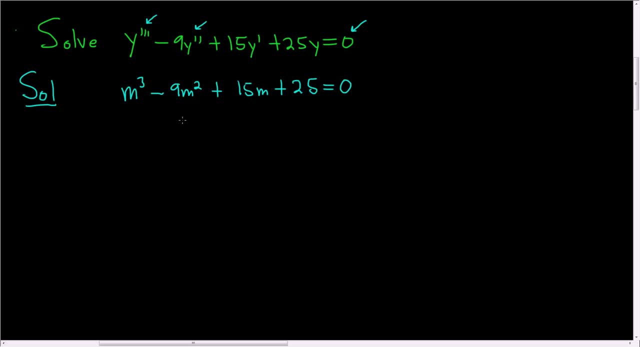 Whenever you have four terms, you should always try to factor by grouping. In this case, it doesn't appear that that will work, So what we'll use is the rational roots theorem. So let's look for the possible rational roots. So, the possible rational roots? well, you look at the last number here. 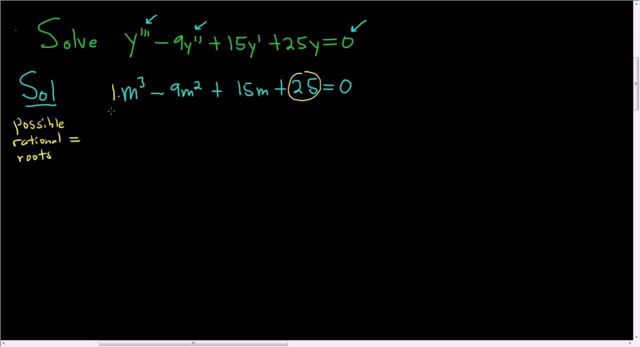 so 25.. And you look at the coefficient here, so one It's always the last over the first. So the factors of 25 are plus or minus one, plus or minus five, and then plus or minus 25.. And then you divide by the. 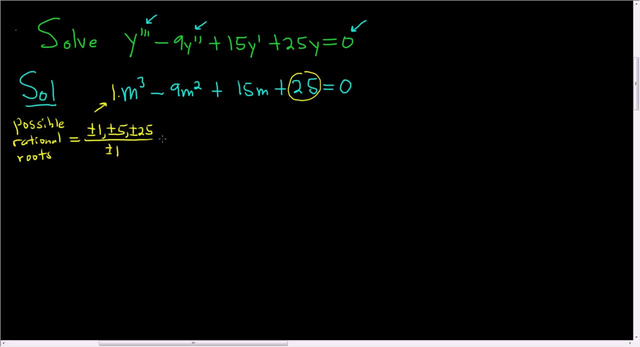 factors of this guy here. so plus or minus one. So in this case the possible rational roots are: let's see: one over one is one, five over one is five and 25 over one is 25.. So these are the. 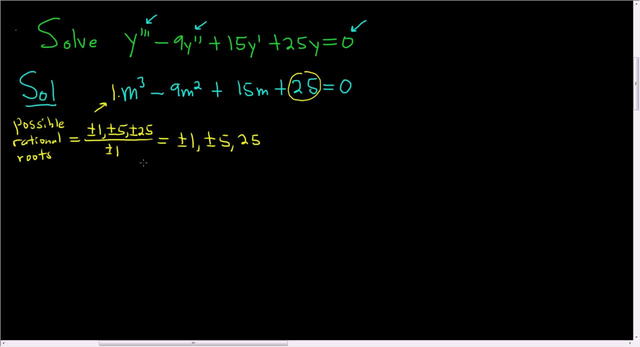 possible rational roots. Now what we do is we start checking them. So let's check one. And so to check one, we use synthetic division, We write the one down and we write the funny box, and then we write the coefficients of 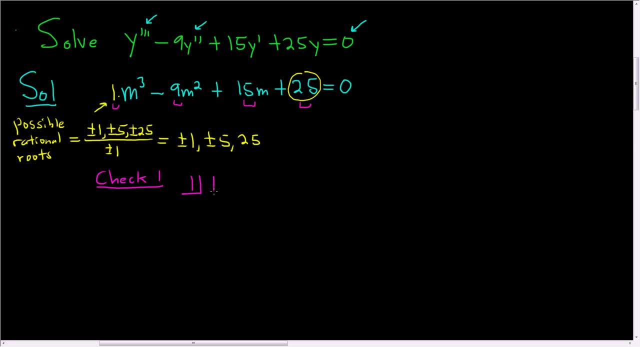 the characteristic equation. So in this case it's one negative nine, 15, and then 25.. Then you draw a line and say, okay, take this number and bring it down. so one One times one is one, and 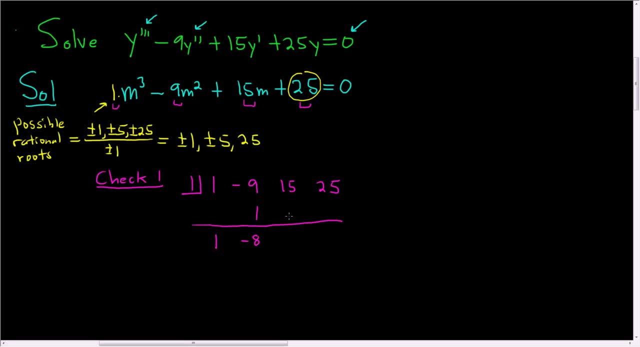 then you add, so you get negative eight, And then negative eight times one is negative eight. And then you add: so you get seven. Seven times one is seven. Oh no, we got 32.. So one is not a root, One is not a root. So when is it a? 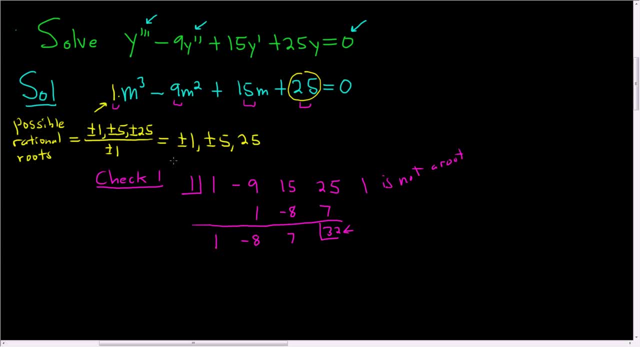 root. Whenever you get zero here, that's a good sign, because you know that one is a root of the original equation. So the next choice, the natural choice to check, is negative one. Let's hope this works. So let's check negative one. 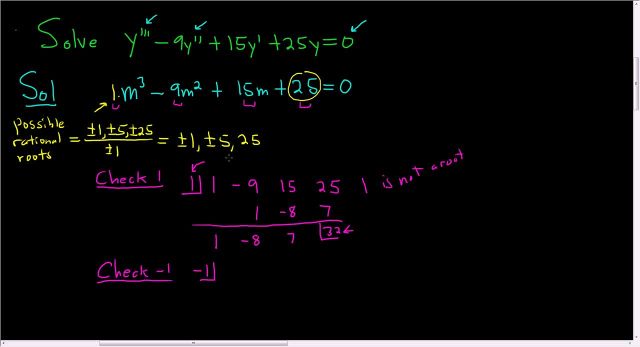 So here we have negative one, And then again one negative, nine, 15,, 25.. So one negative, nine, 15, and then 25. And you just keep doing this and cross your fingers. So let's see One. we write. 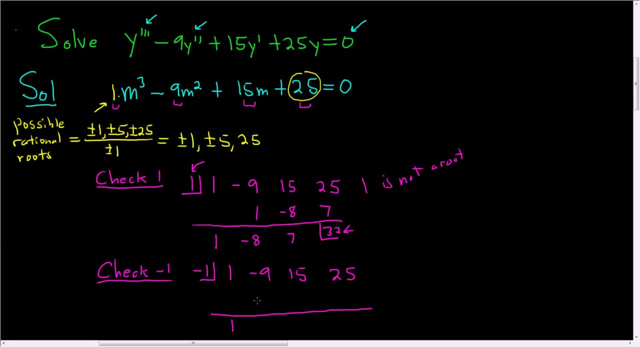 that down. So always bring that first one down. One times negative one is negative one. If we add, we get negative 10.. Negative 10 times negative one is 10. If we add, we get 25. And 25 times. 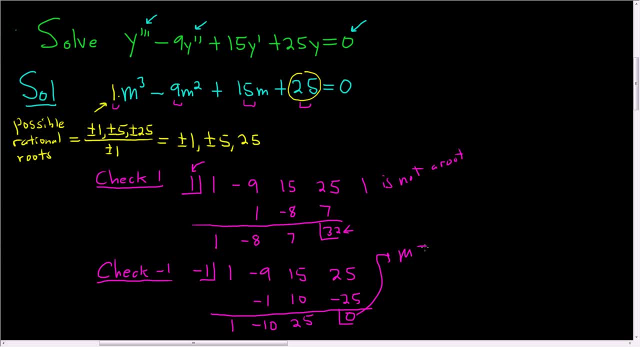 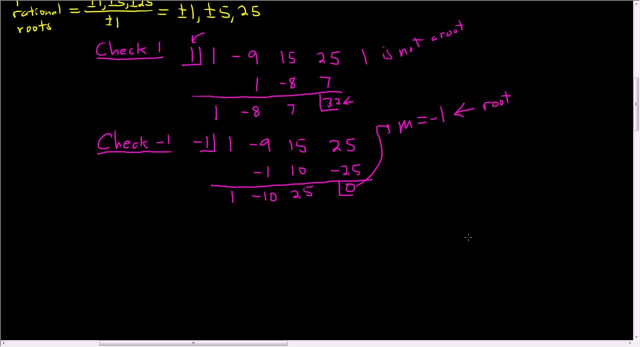 that we get zero, We can rejoice, because this means that m equals negative one. This guy is a root. So to finish, we started with an equation of degree three. So we take this piece and we write it as an equation of degree two. So it's one times m squared, which is just m squared minus 10 times. 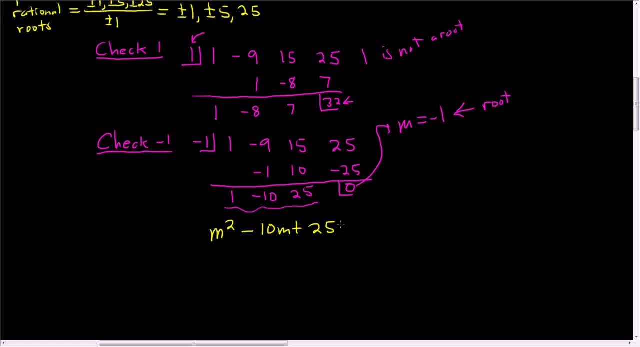 m plus 25, and that's equal to zero. This looks like it factors. looks like m minus five and that's m minus five. Yep, because negative five m and negative five m give you the middle piece, And negative five times negative five is positive 25.. And m times m is m squared. So this is really m. 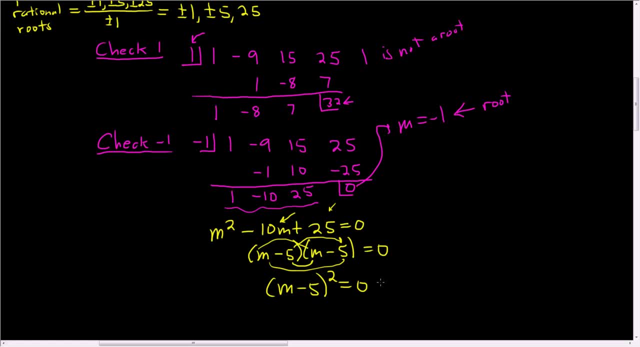 minus five, quantity squared equal to zero. So that tells us that m equals five is a root of multiplicity two. right, Because it appears twice. we have m minus five, m minus five. So we have two roots. m equals negative one, it's a root of multiplicity one. And m equals five is a root of. 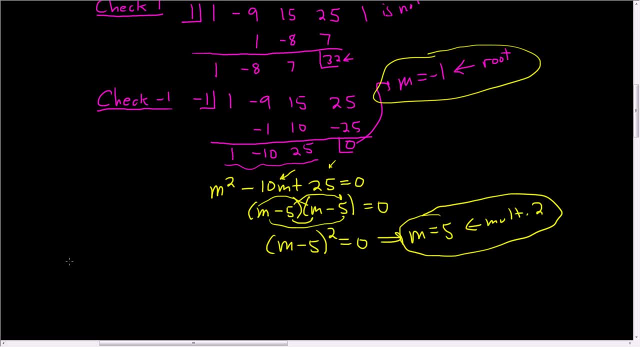 multiplicity two. So let's go ahead and write the final answer down. Let's start with the negative one. So y is equal to c one, e to the negative x. right, you just put the root there plus c two.